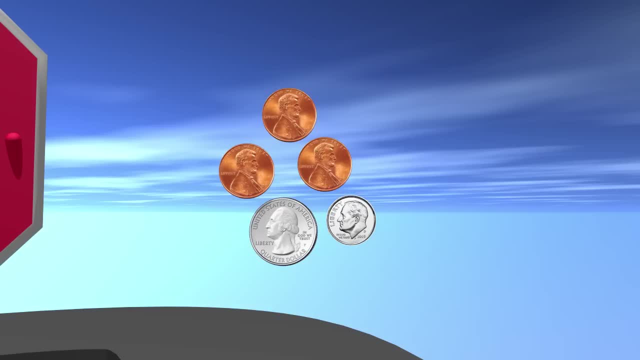 Here we have some coins and we need to count them to get past this checkpoint. When we count money, it is a good idea to start counting the coin with the most value. Here we have a quarter, a dime and three pennies. Which of these coins has the most value? 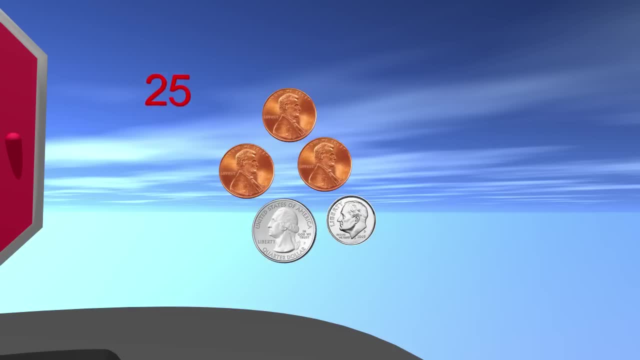 The quarter has the most value And we know it is worth 25 cents. Now we have a dime and three pennies left. Which one is worth more, the dime or the pennies? The dime is worth more, since it is worth 10 cents. 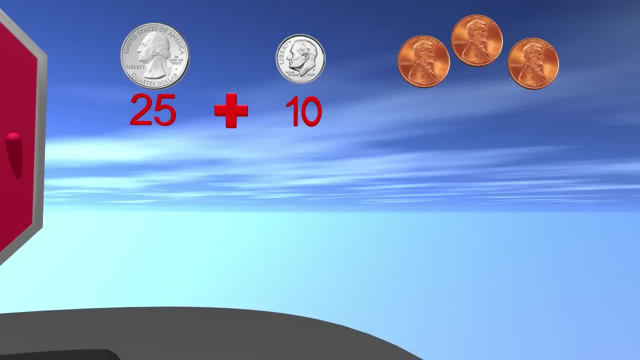 We know that each of these pennies is worth 1 cent and there are three of them. so we know these pennies are worth 3 cents. So we have 25 plus 10 plus 3.. Adding this up might seem hard, but we can do it by breaking it down. 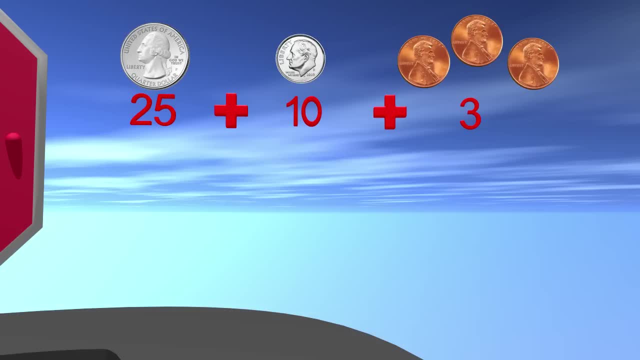 into smaller parts. To start, let's just add the 25 and the 10 together. So 25 plus 10 is 35.. Now we just need to add the 3.. So 35 plus 3 gives us 38.. 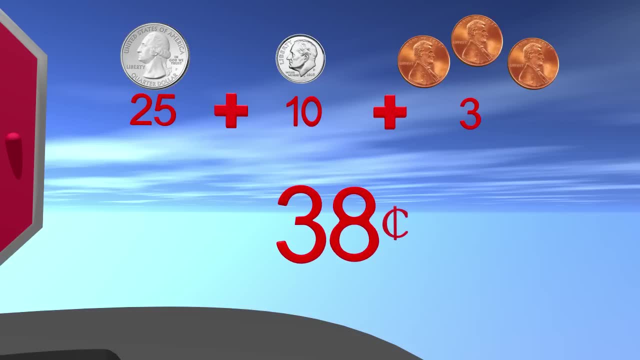 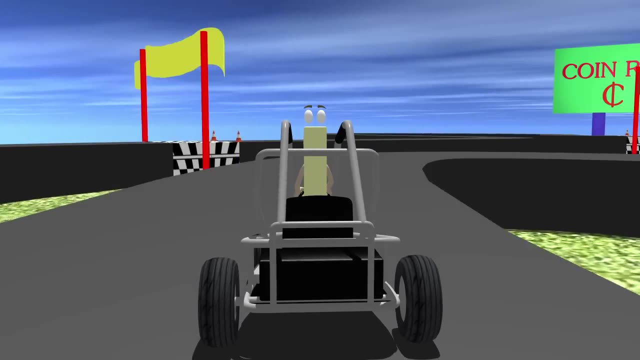 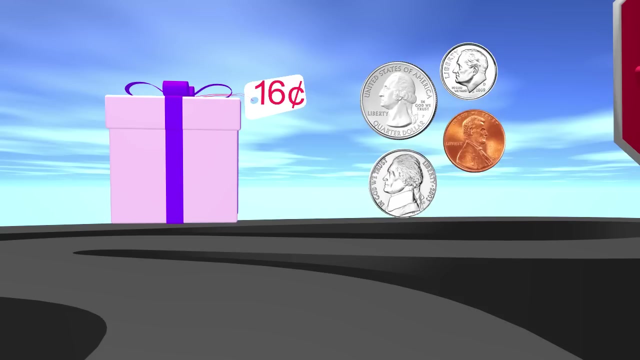 The answer is 38.. Great job, We have 38 cents. Okay, let's move on. We are at another checkpoint and we need to solve another problem to get past Here. we have a gift that costs 16 cents. We have some coins and we need to get exactly 16 cents to buy this gift. 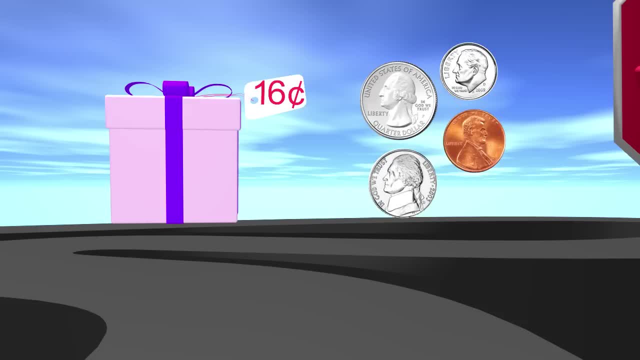 How can we get 16 cents using these coins? Well, we do not want to use the quarter because it is worth 25 cents and that is too big to get exact change. Let's start with the dime. We have a dime that is worth 10 cents. 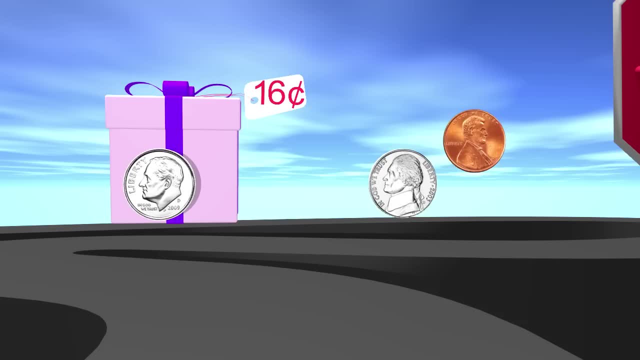 But we still do not have 16 cents. What other coins can we use to get the 16 cents? If you said the nickel and the penny, you are correct. We now have 10 plus 5 plus 1, which equals 16 cents. 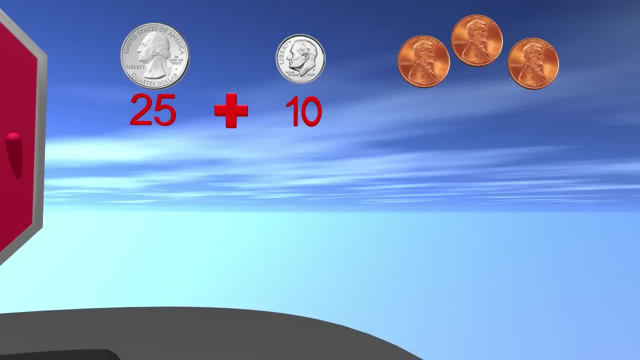 We know that each of these pennies is worth 1 cent and there are three of them. so we know these pennies are worth 3 cents. So we have 25 plus 10 plus 3.. Adding this up might seem hard, but we can do it by breaking it down. 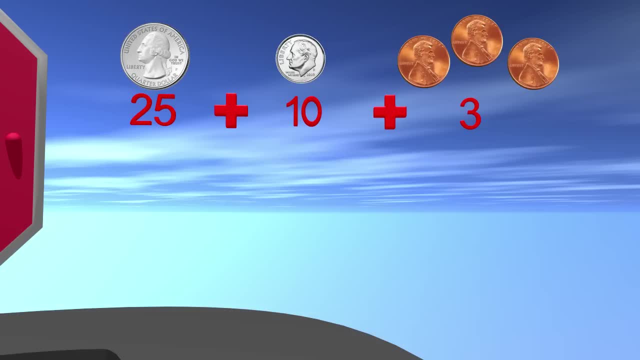 into smaller parts. To start, let's just add the 25 and the 10 together. So 25 plus 10 is 35.. Now we just need to add the 3.. So 35 plus 3 gives us 38.. 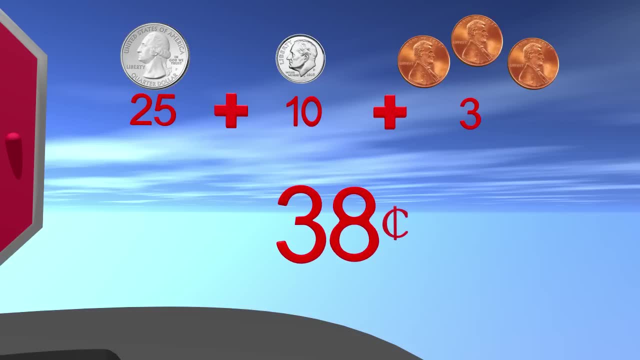 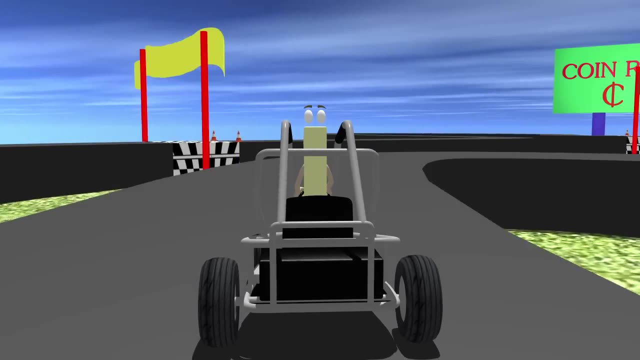 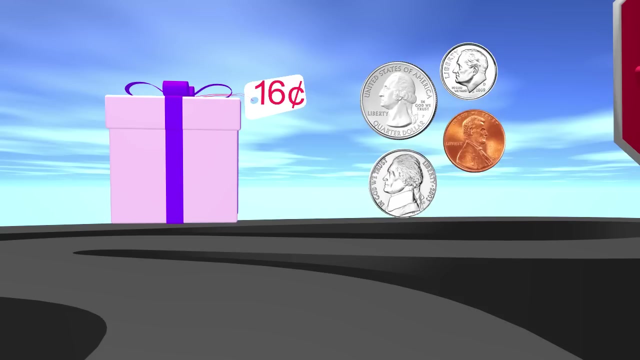 The answer is 38.. Great job, We have 38 cents. Okay, let's move on. We are at another checkpoint and we need to solve another problem to get past Here. we have a gift that costs 16 cents. We have some coins and we need to get exactly 16 cents to buy this gift. 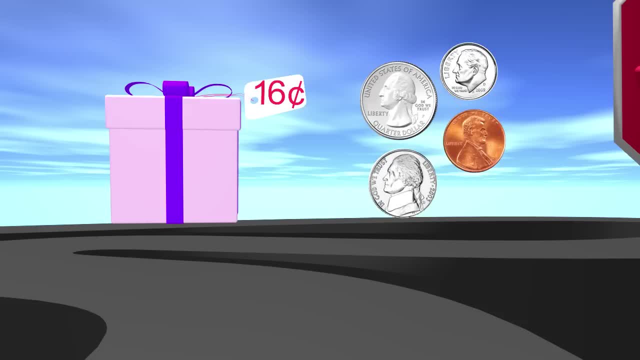 How can we get 16 cents using these coins? Well, we do not want to use the quarter because it is worth 25 cents and that is too big to get exact change. Let's start with the dime. We have a dime that is worth 10 cents. 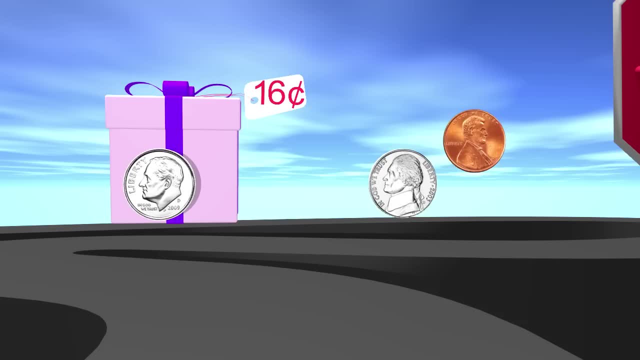 But we still do not have 16 cents. What other coins can we use to get the 16 cents? If you said the nickel and the penny, you are correct. We now have 10 plus 5 plus 1, which equals 16 cents. 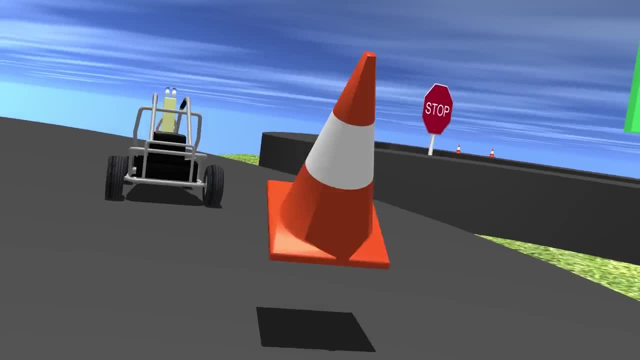 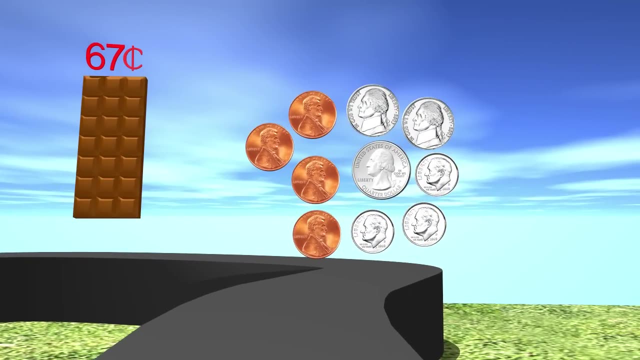 Great job, guys. Okay, we are at our last checkpoint and this problem is a little bit harder. We have a candy bar here that costs 67 cents. On the right side we have a bunch of change. Do we have enough change to buy this candy bar? 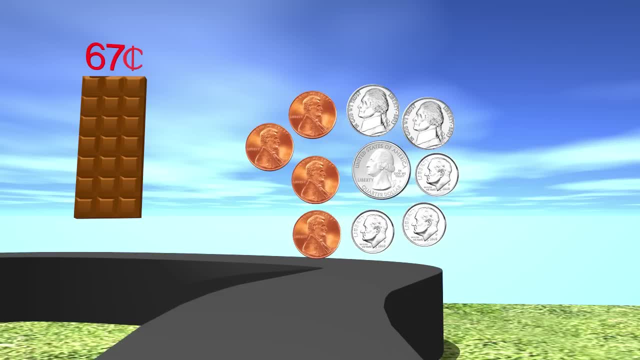 Take a minute and look at this. Now that you have looked at it, let's go through it together. First, we look at the coin with the biggest value, which is the quarter. This is worth 25 cents, so we put down the 25.. 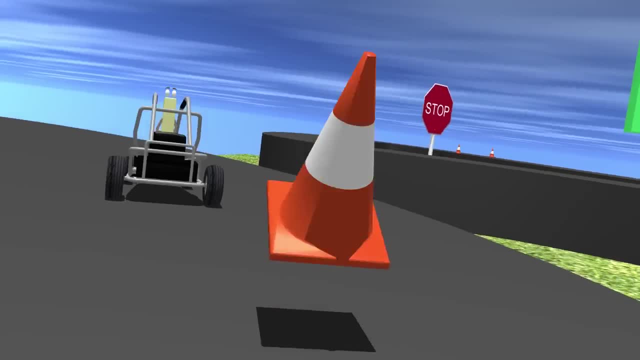 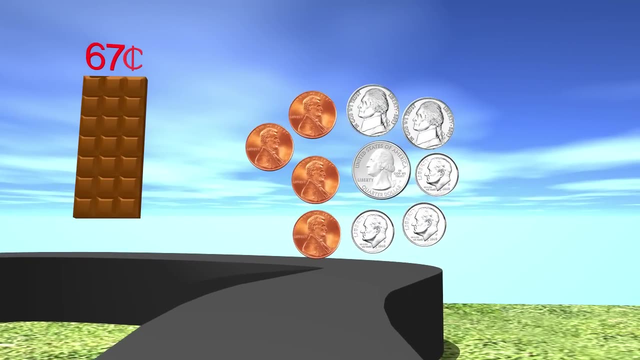 Great job, guys. We are at our last checkpoint. This problem is a little bit harder. We have a candy bar here that costs 67 cents. On the right side we have a bunch of change. Do we have enough change to buy this candy bar? 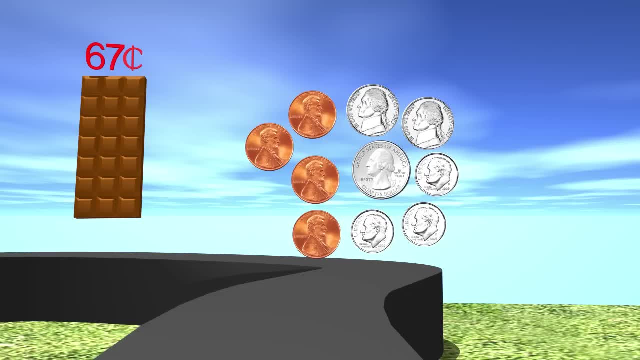 Take a minute and look at this. Let's see. Now that you have looked at it, Let's go through it together. First, we look at the coin with the biggest value, which is the quarter. This is worth 25 cents, So we put down the 25.. 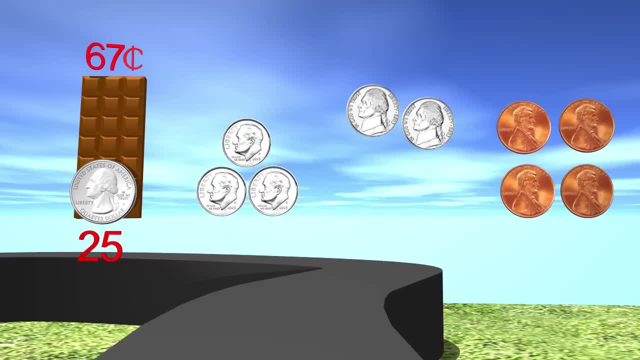 Now we move to the dime, which is worth 10 cents. How much are these dimes worth 30 cents? Great job. Next, we have two nickels. How much are these two nickels worth 10 cents? Great job again. 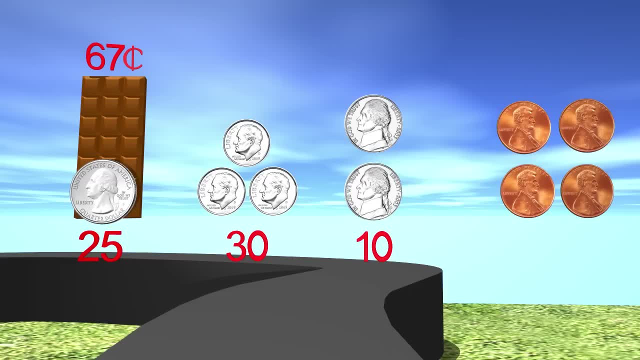 Last of all, we look at the pennies. How much are these pennies worth? 4 cents, Great job. So we have 25 plus 30 plus 10 plus 4.. To add these together can be tricky, So I think we will count on to find the answer. 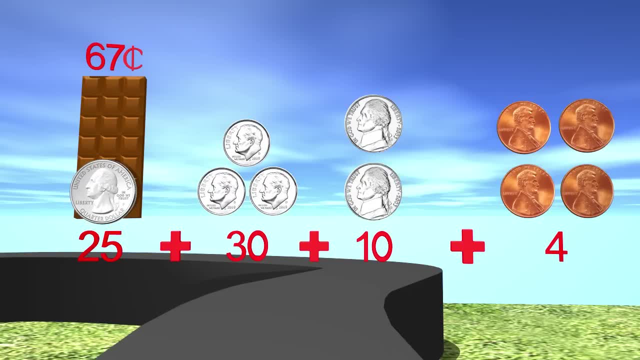 Looking at the quarter, we have 25 cents. Now to count on using our dimes, we count by 10.. We have 3 cents, 35,, 45,, 55. So the quarter and the dimes added together give us 55 cents. 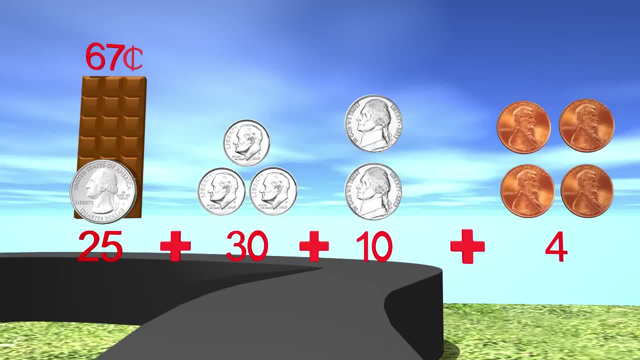 Now we have the nickels to count, So we will count by 5's. So 55 plus 5 is 60. And another nickel gives us 65. We just have the pennies left and they are easy to count. So we get 66,, 67,, 68,, 69. 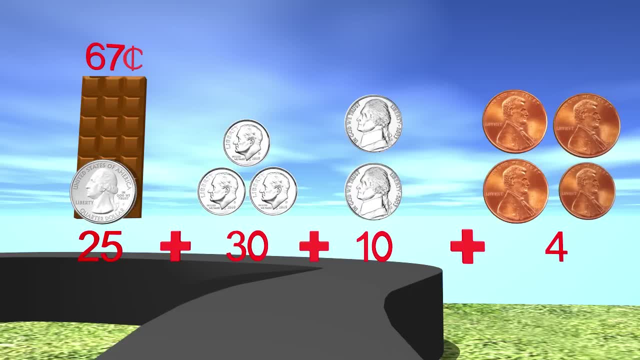 So we have the nickels to count, So we will count by 5's. So 55 plus 5 is 60.. 69.. Great job, guys. Ok, we have 69 cents in all and the candy bar costs 67 cents. 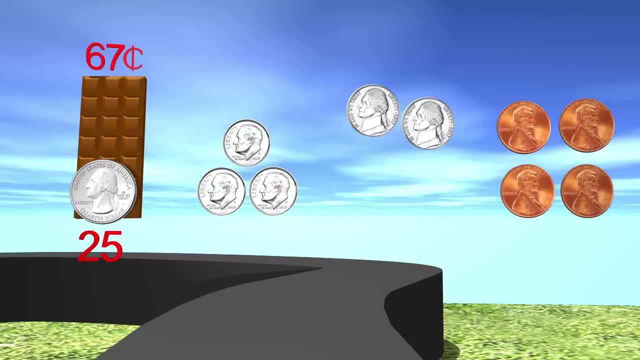 Now we move to the dime, which is worth 10 cents. How much are these dimes worth 30 cents? Great job. Next, we have two nickels. How much are these two nickels worth 10 cents? Great job again. 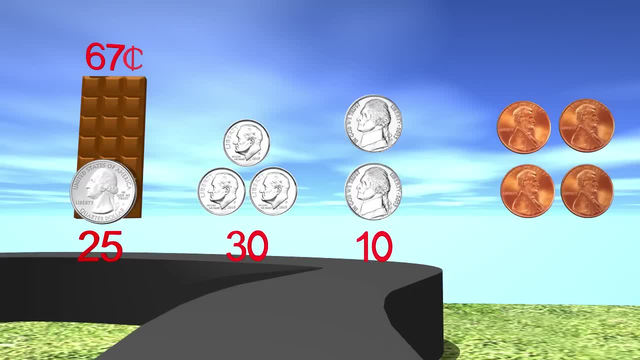 Last of all, we look at the pennies. How much are these pennies worth? 4 cents, Great job. So we have 25 plus 30 plus 10 plus 4.. To add these together can be tricky, so I think we will count on to find the answer. 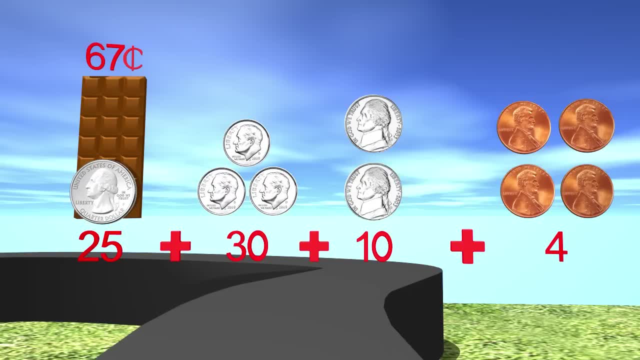 Looking at the quarter, we have 25 cents. Now to count on using our dimes, we count by 10.. We have 35.. 45., 45., 55. So the quarter and the dimes added together give us 55 cents. 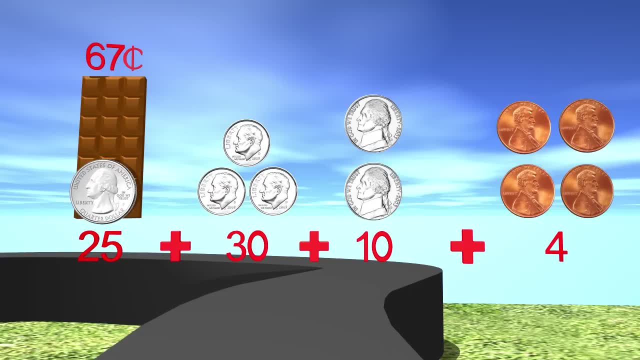 Now we have the nickels to count, so we will count by fives. So 55 plus 5 is 60. And another nickel gives us 65. We just have the pennies left and they are easy to count. So we get 66,, 67,, 68,, 69, and 60. 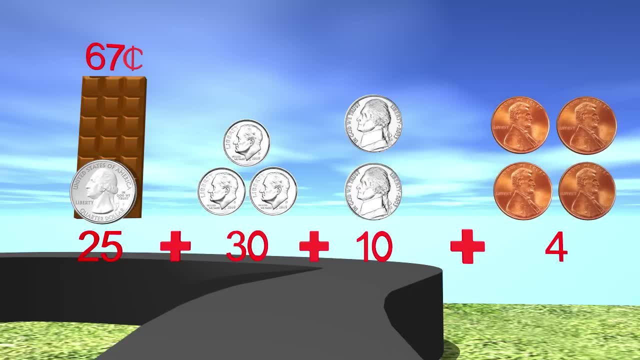 So we have 65,, 65,, 65, and 60. So we have 65,, 65,, 65, and 60. So we have 69.. Great job, guys. Okay, we have 69 cents in all and the candy bar costs 67 cents. 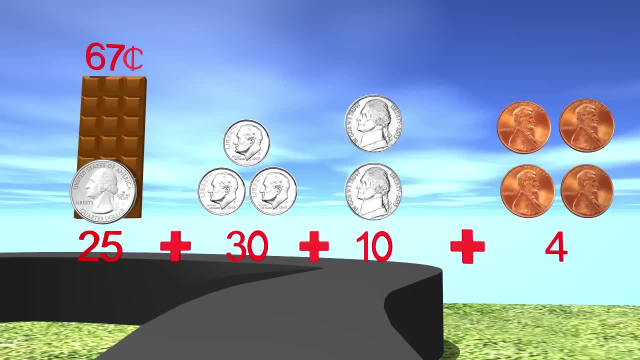 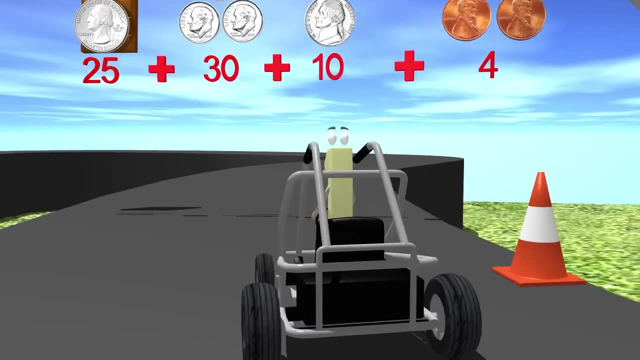 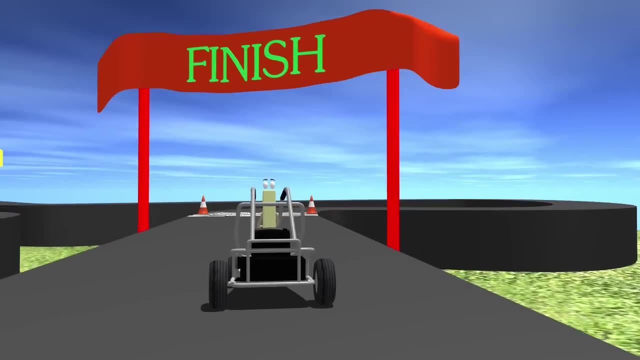 So do we have enough money to buy the candy bar? Yes, we do have enough money. Alright, guys, let's finish this race. Woohoo, Alright, thanks for all your help, guys. Okay, we'll see you next time. 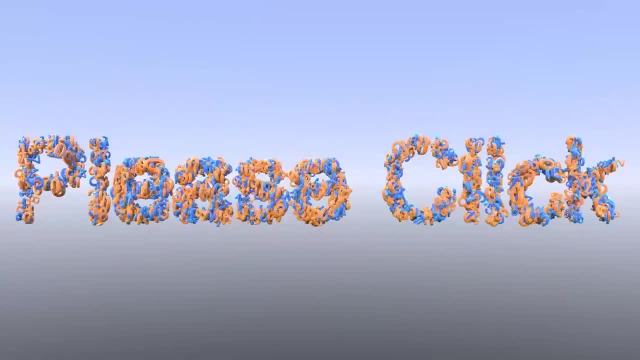 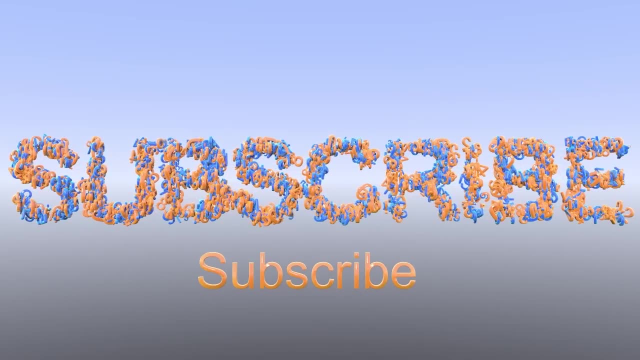